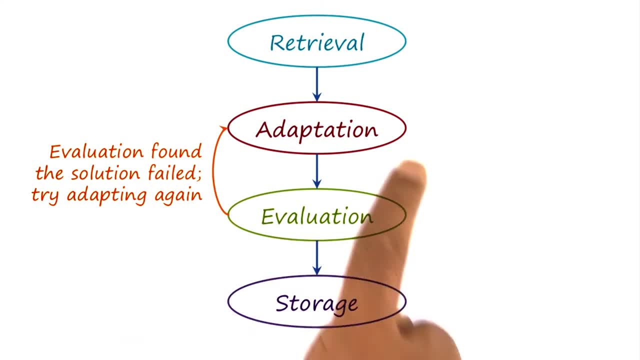 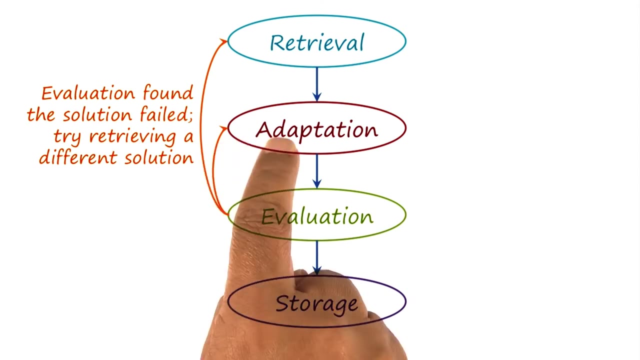 an example: if the evaluation of the candidate solution that adaptation had produced fails, then instead of abandoning that particular case, we might want to try to adapt it again. Alternatively, if we have tried to adapt the same case several times but we just cannot adapt it, we might want to abandon that case and 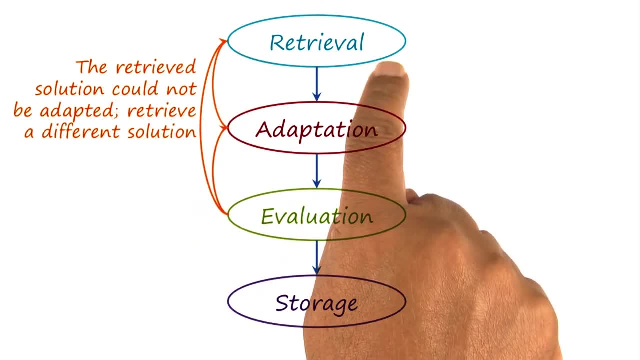 try to find a different case from the case memory. Here is another possibility. Suppose that we retrieve a case from memory and we try to adapt it, but we are unable to adapt it to meet the requirements of the new problem. In that case we might want to abandon. 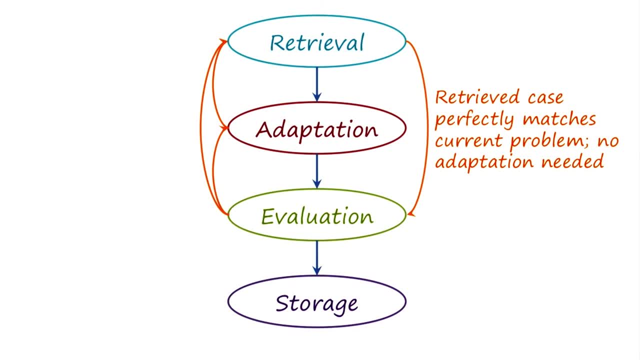 the case and try to retrieve a new one. Here is yet another possibility. Let us suppose that we retrieve a case from memory and it exactly matches the new problem. In that case, no adaptation needs to be done and we can jump down through the evaluation. In fact, this is what happened when we were discussing 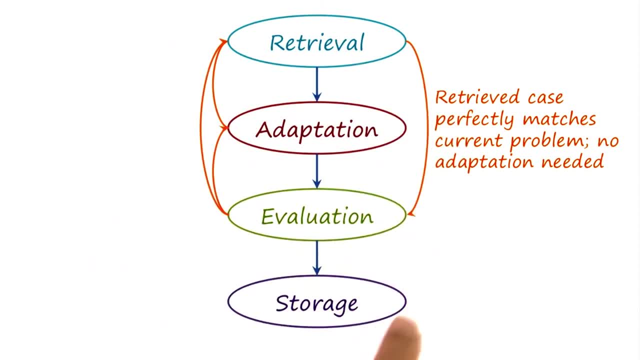 the KNN method. In this way, we can see that there are many ways in which this process need not necessarily be linear. So, Ashok, earlier you said that if the evaluation shows that the new solution is good, then we should store it. 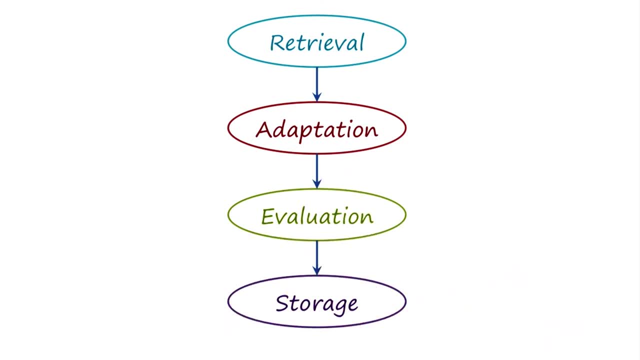 If the evaluation shows that the new solution is not good, we should try adapting again or we should try retrieving again. But what about evaluation showing that the new solution is not good? Should we ever store those Indeed? sometimes storing failed cases is also very useful. Failed cases can. 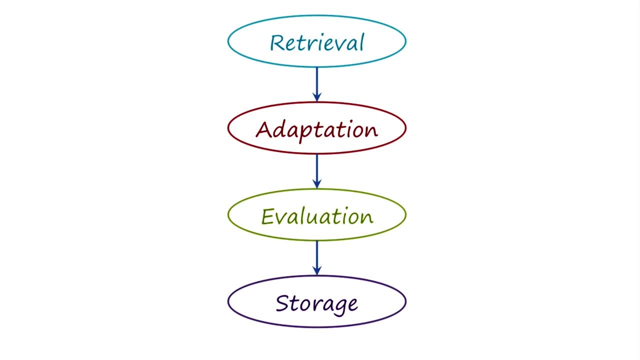 help us anticipate problems. So imagine that you're given a new problem and you retrieve from your case memory a failed case. That failed case can be very useful because it can help you anticipate the kinds of problems that will occur in solving the new problem. 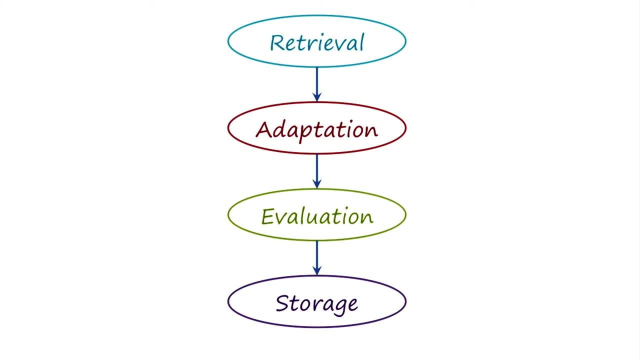 So that reminds me of another example from our file input problem. One thing I've encountered a lot when I'm doing file input is that if you read too far in the file then the program will crash and it will give you an error. It will always. 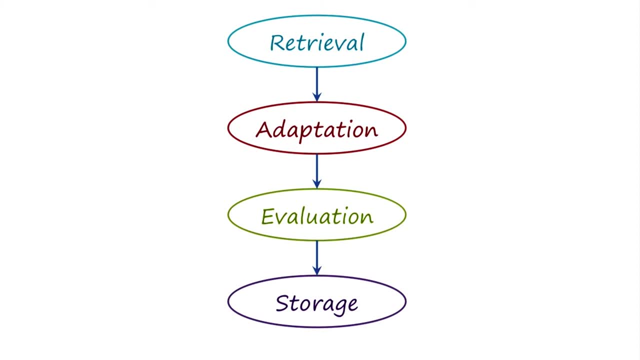 give you the same error, and it's a very common problem because different languages do file input slightly differently. So in my mind I must have cases of the different ways that it's failed in the past so I can anticipate those and do it correctly in the future.